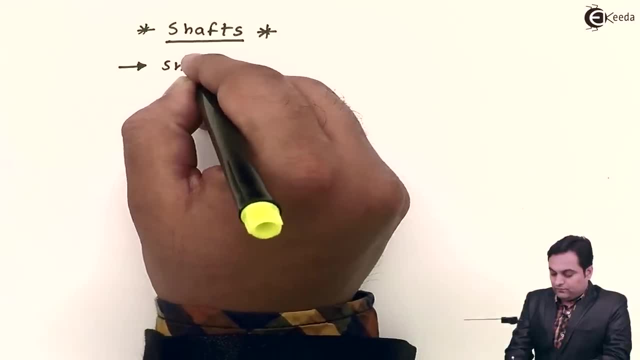 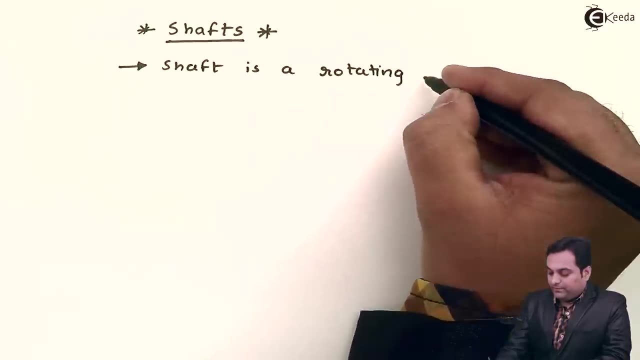 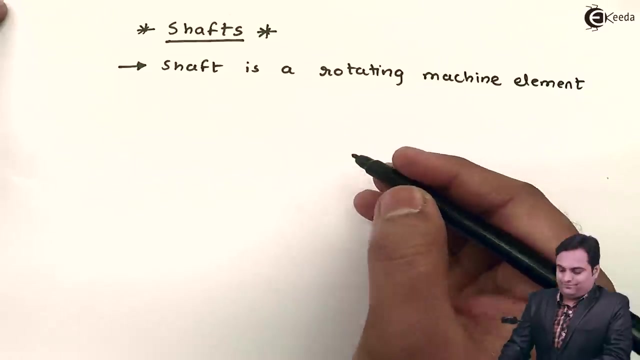 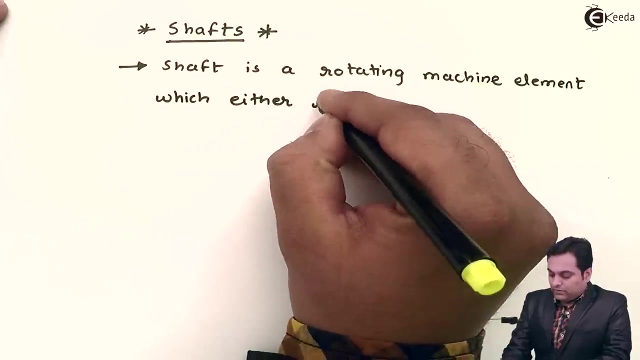 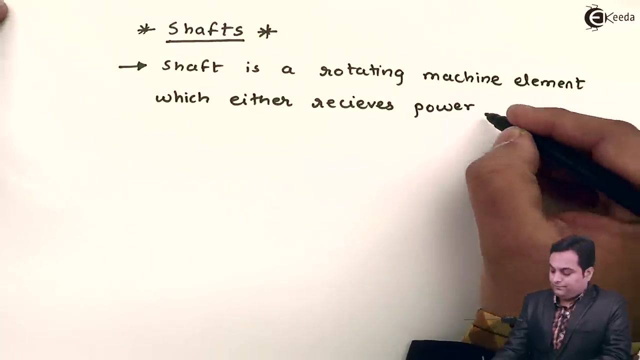 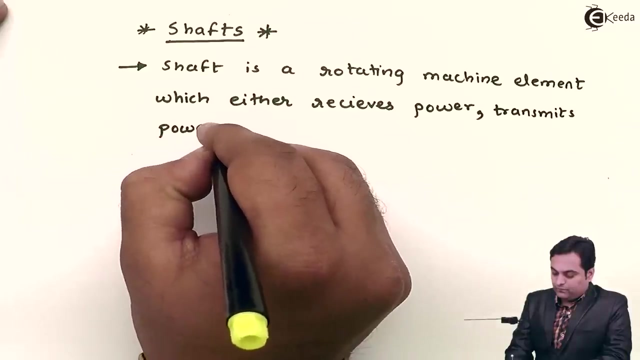 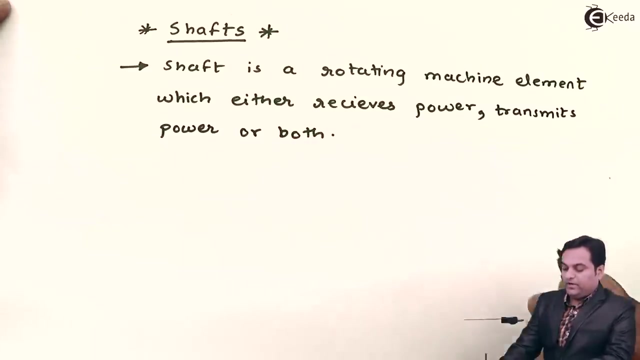 Shaft is a rotating machine element which either receives power, transmits power, or both, That is, it would receiving the power as well as transmitting the power. So here we have the definition of shaft, that it is a rotating machine element which either receives power, transmits power, or both. 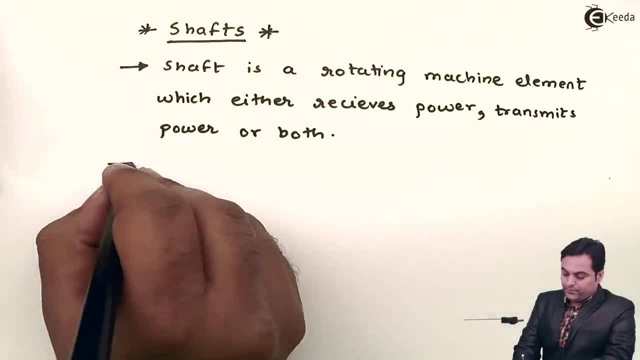 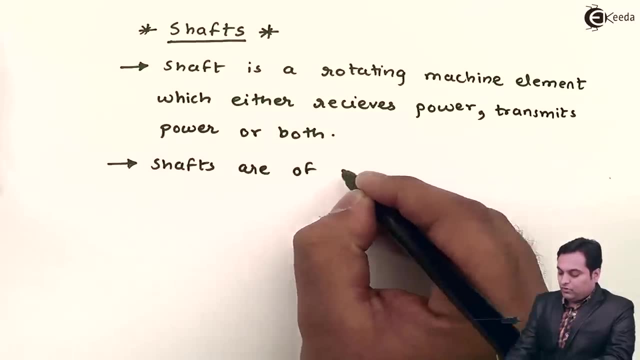 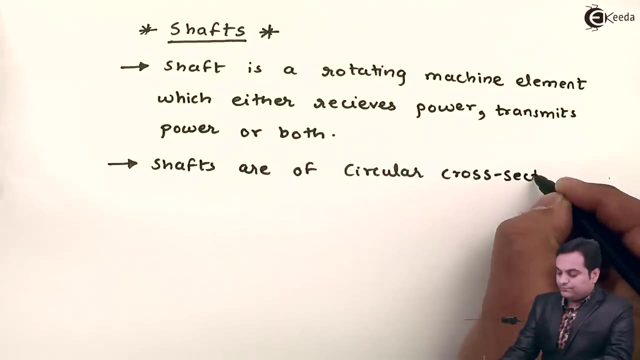 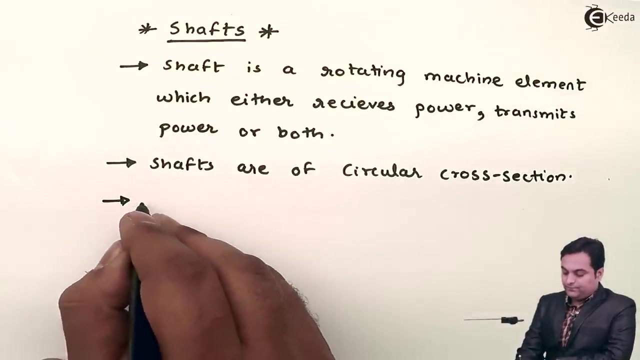 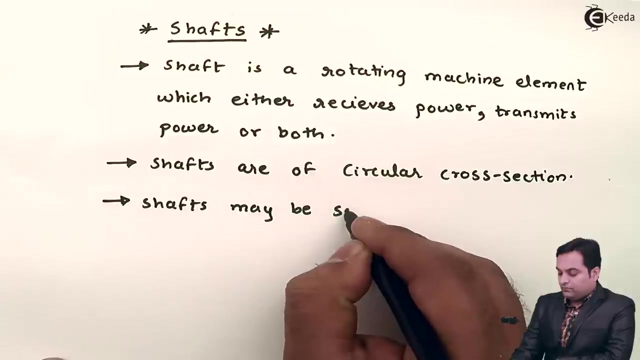 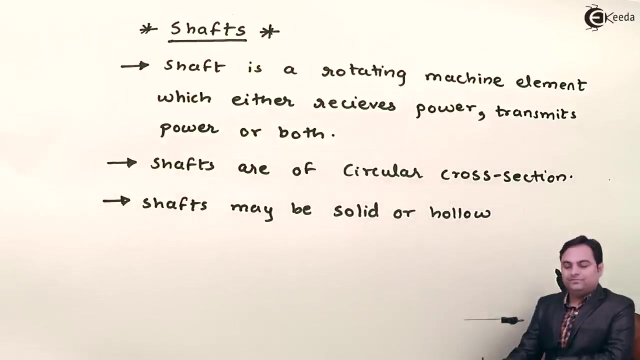 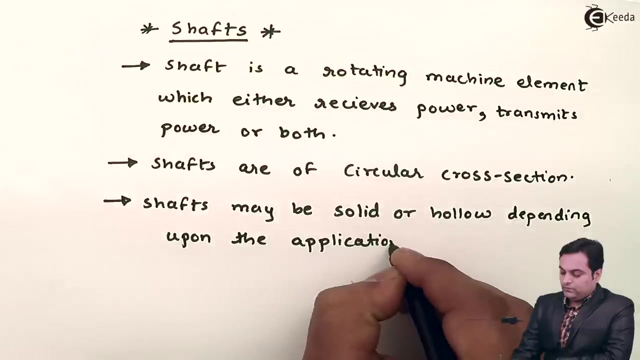 That is, receiving the power and even transmitting it. Now next is shafts are of circular cross section. that is the cross section. the area of the shaft is circular. Next, shafts may be solid, solid or hollow, depending upon the application. That is, we can either use solid shaft or we can use hollow shaft. 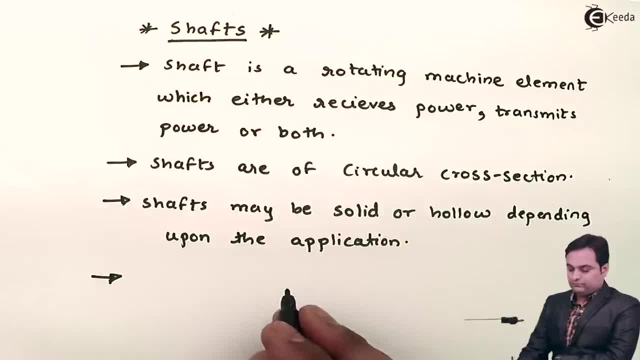 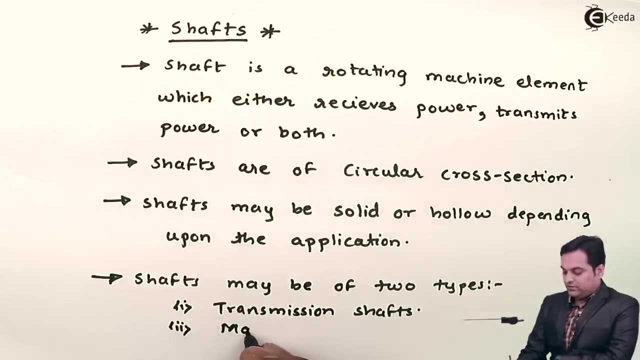 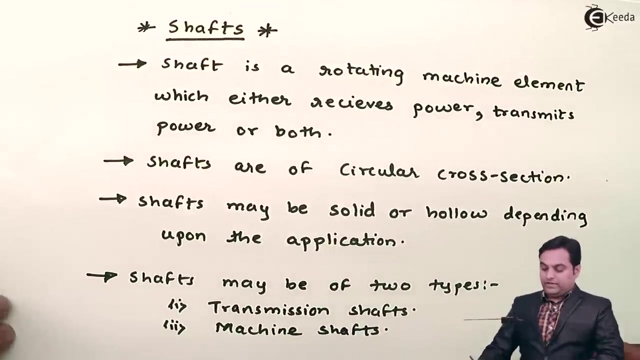 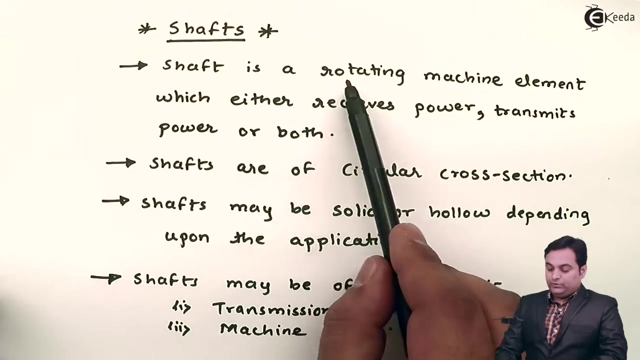 Next, shafts may be of two types, that is, they can be transmission shafts or the second one called as machine shafts. So here I have written a brief description about shafts. First, it is a rotating machine element that receives power, transmits power, or both. 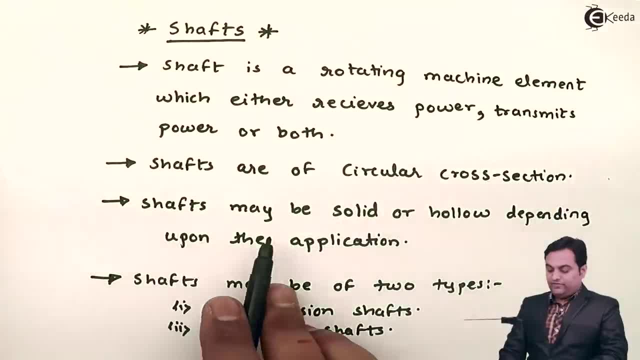 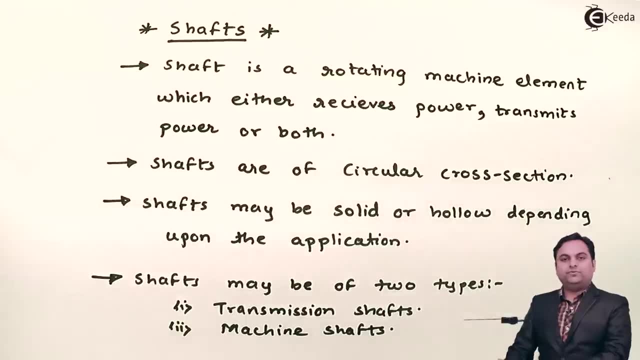 Next, shafts are of a circular cross section. Shafts may be solid or hollow, depending on the application. Shafts may be of two types: transmission shafts or machine shafts. Now I will draw a diagram to explain how similar shafts can be used for machine shafts. 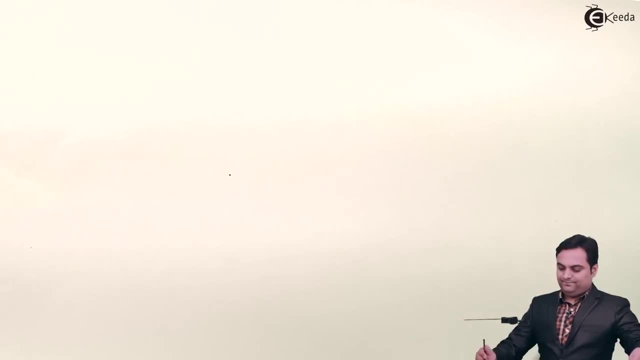 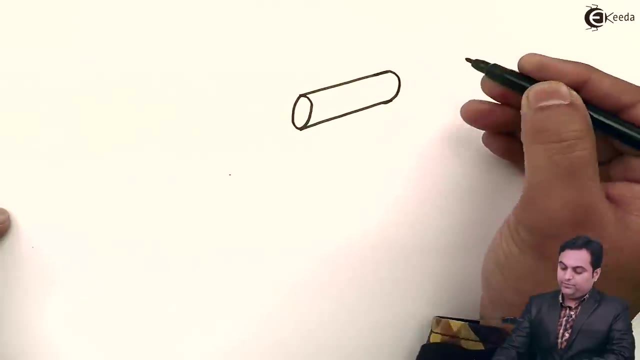 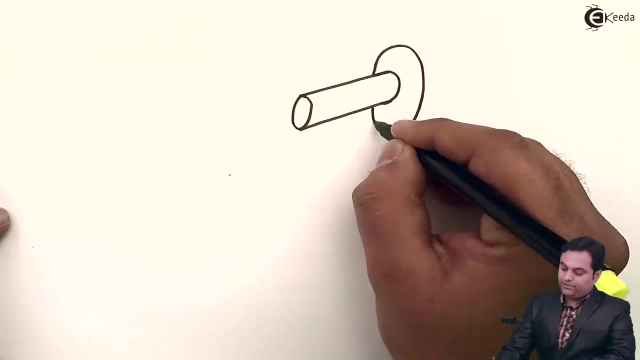 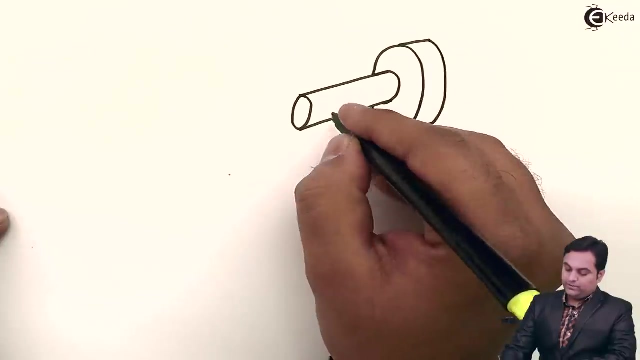 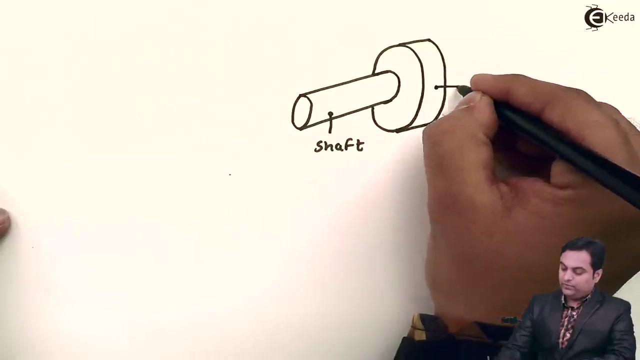 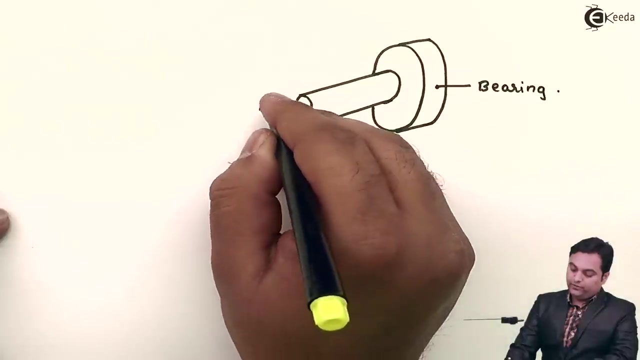 diagram to explain how the shaft looks like shaft is. since it is rotating machine element, it would be supported in some member and that member. it is called as bearing. so here we have a shaft and the member inside which it is supported it is called as bearing. now this shaft would be rotating inside this bearing. so 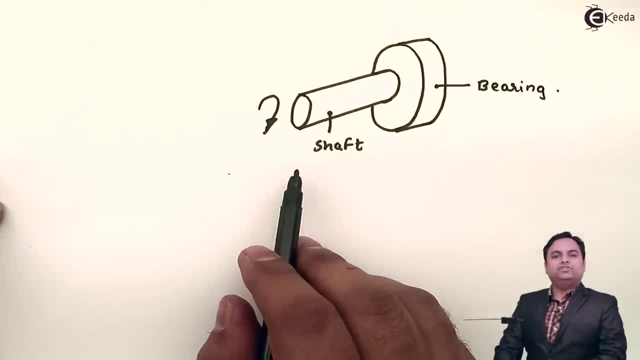 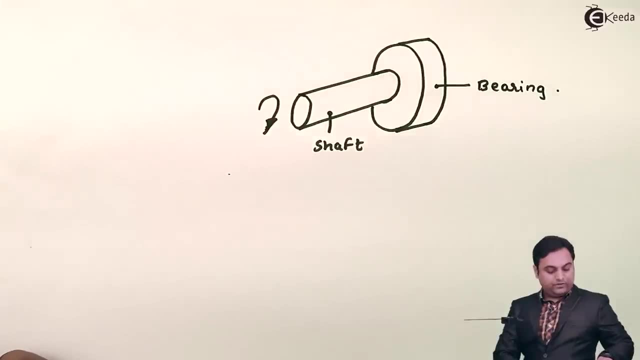 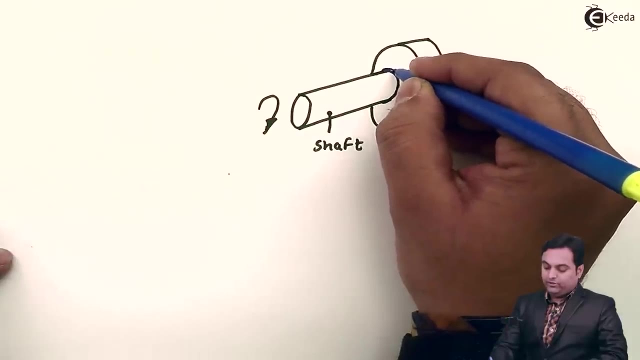 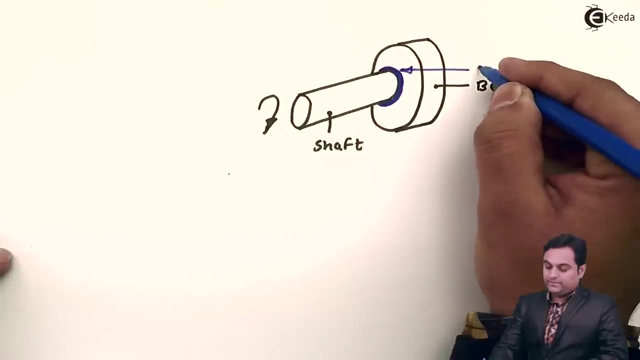 as I have described, that, it is a rotating machine element. so here it will rotate and to support the shaft we have bearing. then the contact between the shaft and bearing it is with the help of oil film, because oil is used as lubrication in the shafts. so here we have an oil film. this in blue it indicates oil film, which 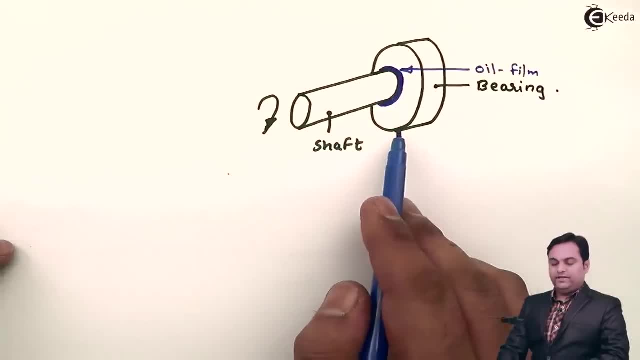 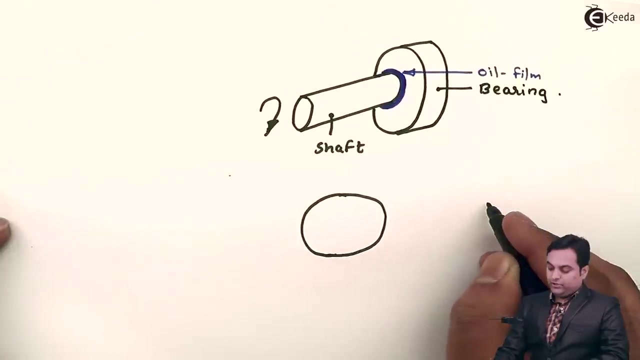 is there for lubrication because both shaft and bearing they are made up of metal. so when the shaft rotates there are chances of metal to metal rubbing. so to avoid that, we are lubricating this shaft. next, as i have told, shafts may be of circular cross section and that circular cross section may be either solid or it. 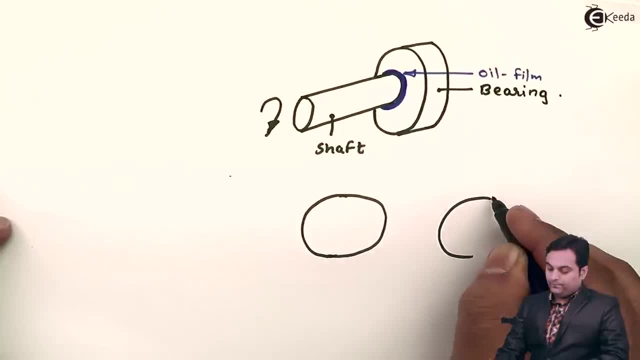 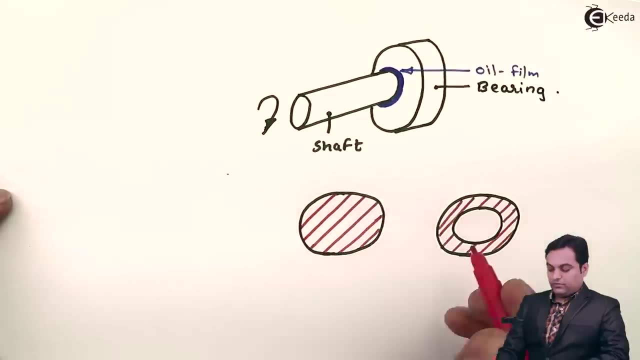 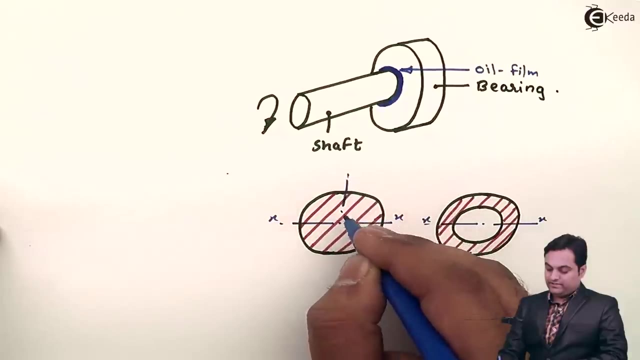 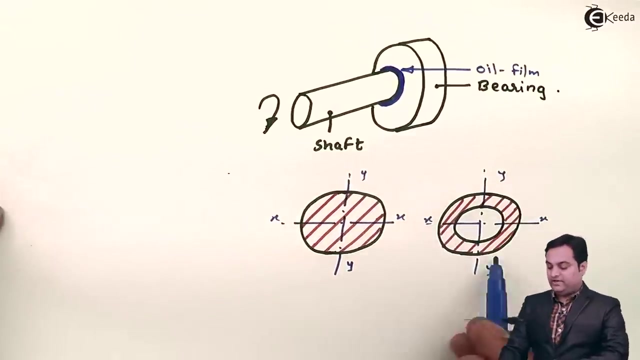 can be hollow. i'll draw the section here. so here is the section of the shaft. i am drawing the axis of this. so now, shafts as i have drawn here it may, it may be of solid cross section or it can be of hollow cross section. so here i have given the example of solid cross section, of shaft and hollow cross section. 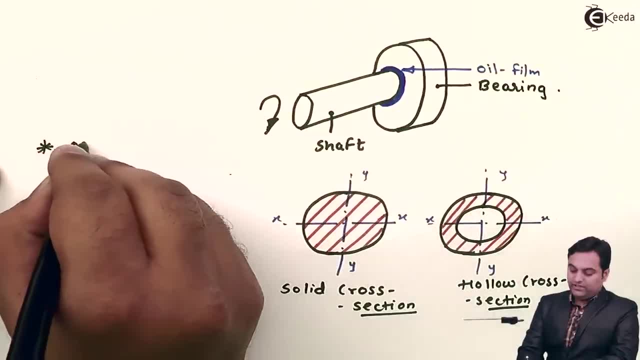 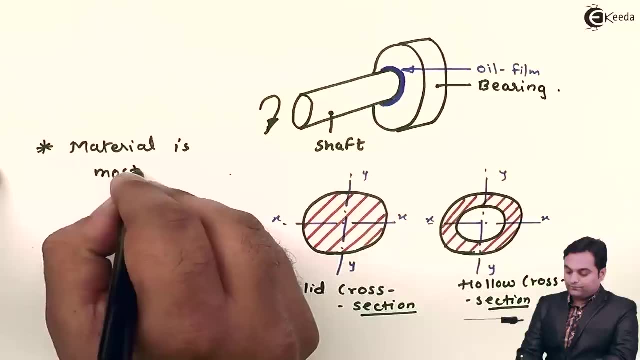 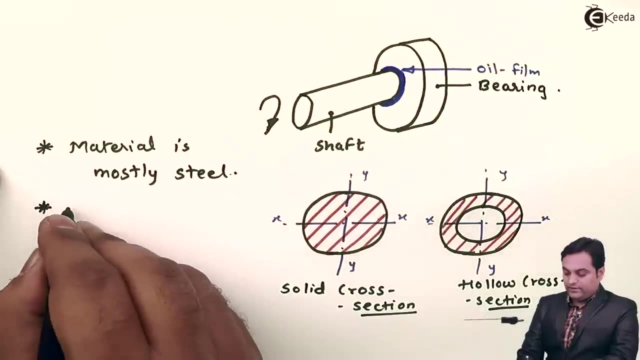 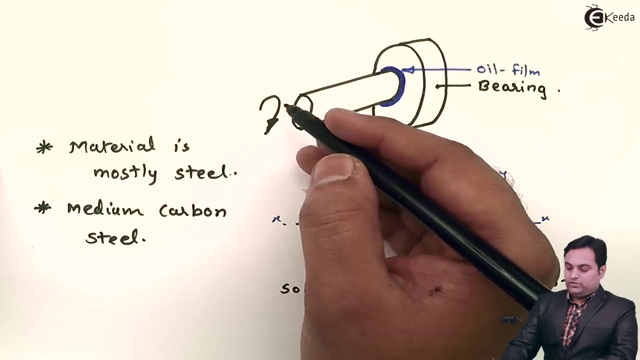 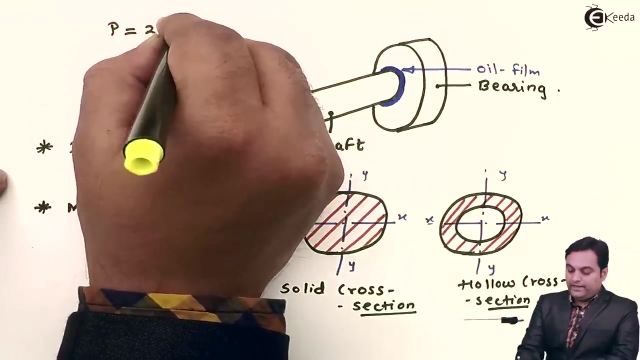 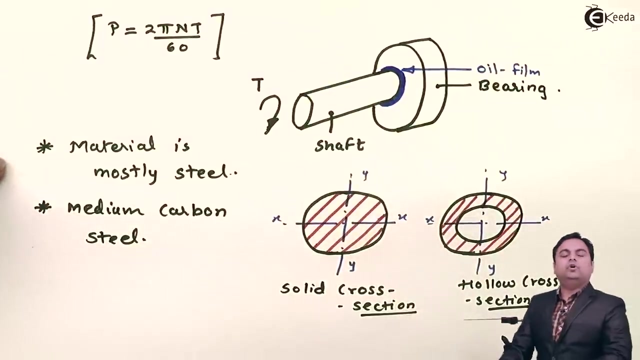 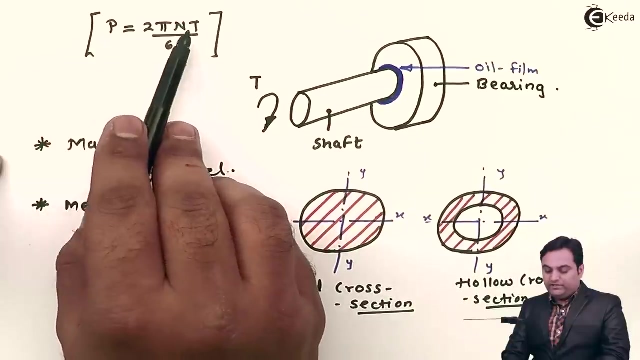 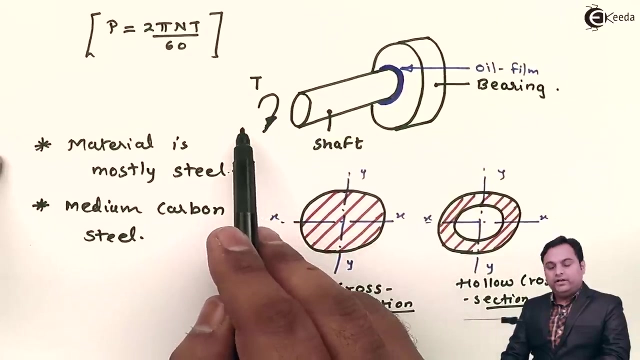 the material used material is mostly steel or we can say in a more precise form, it is medium carbon steel which is used as a material for the shaft. now, when the shaft rotates, we are providing the torque because, since we know that power, it is equal to 2 pi N T upon 60. so the power consumed by the shaft or the power transmitted by the shaft, it can be found out by using this formula and, as we can see, power and torque, they are directly proportional. so this torque, that is that we can say rotation, it produces power, or either the shaft consumes this power. next, after this, we are 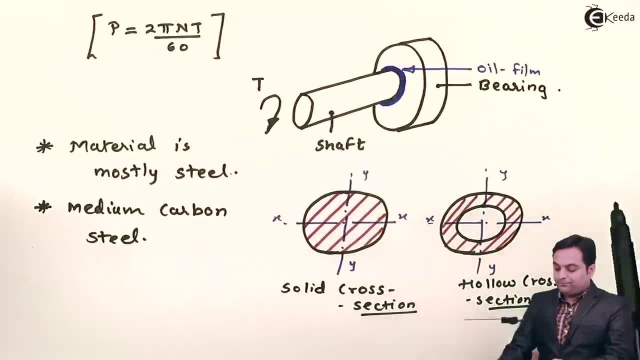 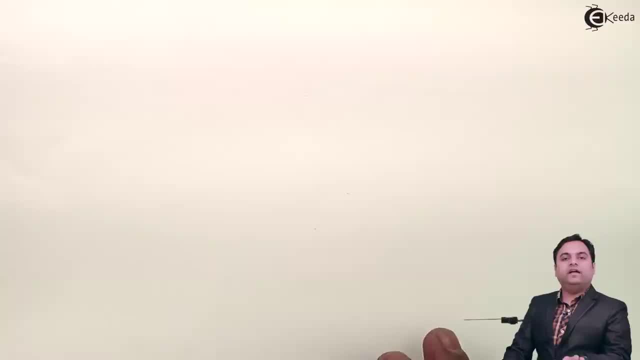 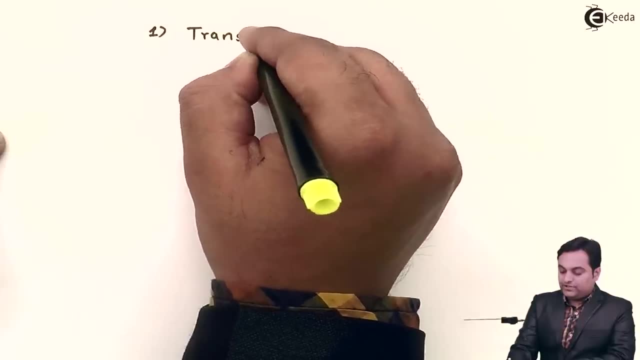 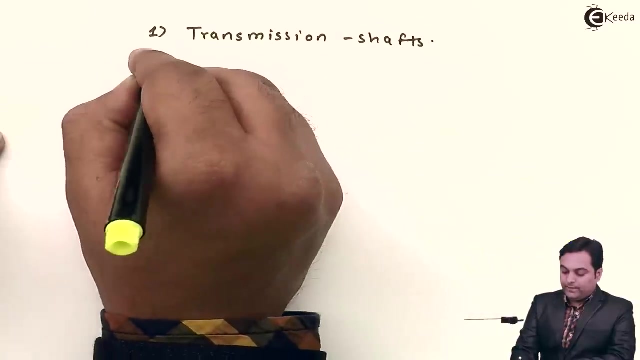 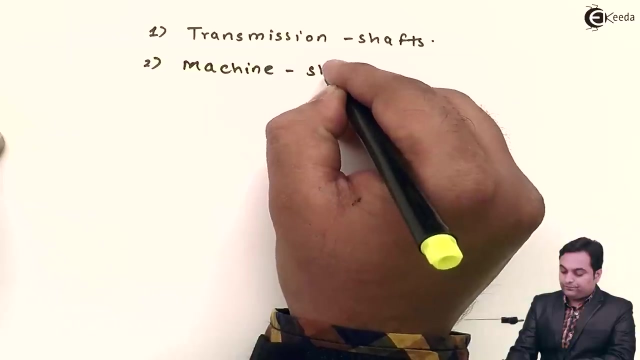 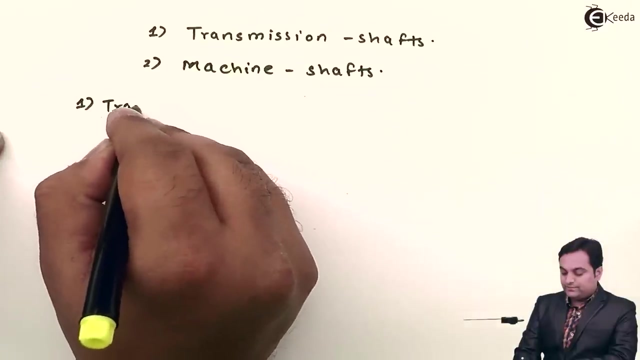 power, or either the shaft consumes this power next, after this, Now shafts. as I have told, there are two types. the first one, it is called as transmission shafts, and the second one, it is called as machine shafts. now, when we are talking about the first one, that is, transmission shafts, 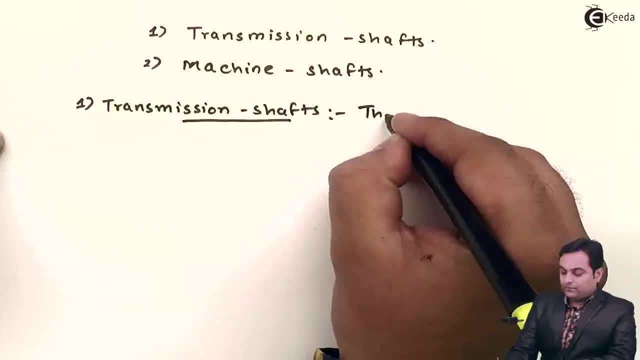 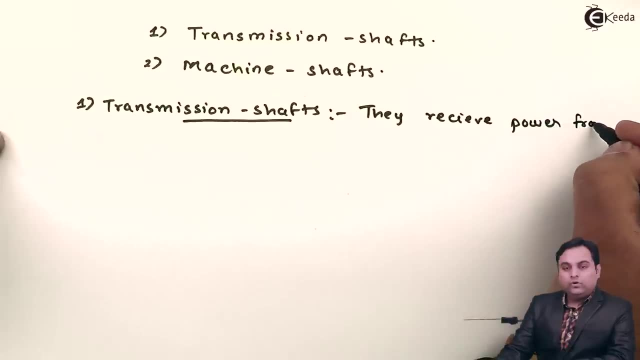 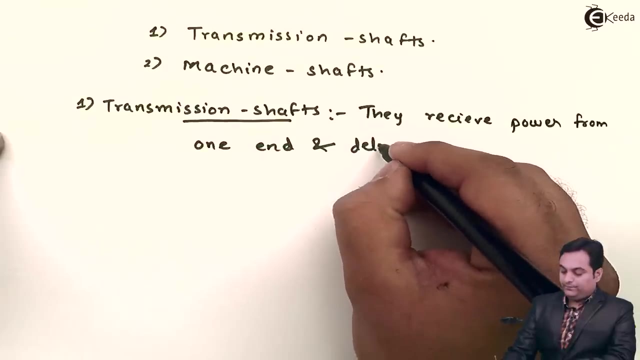 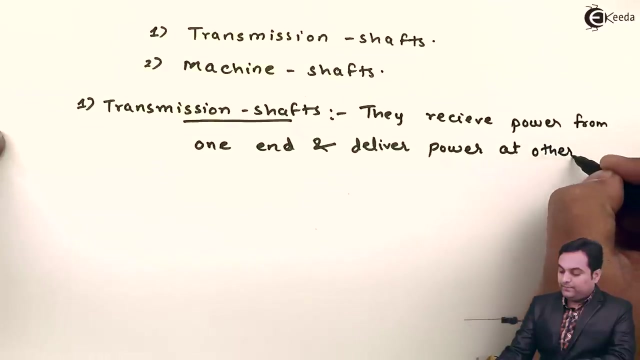 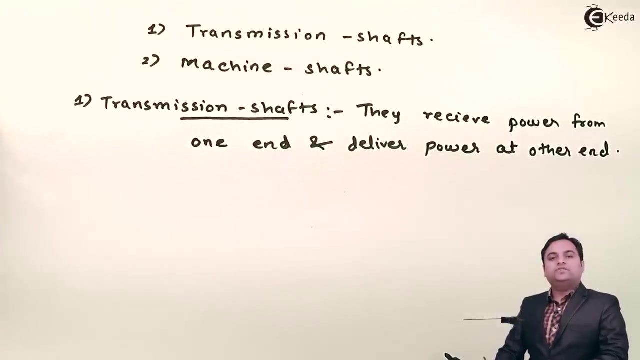 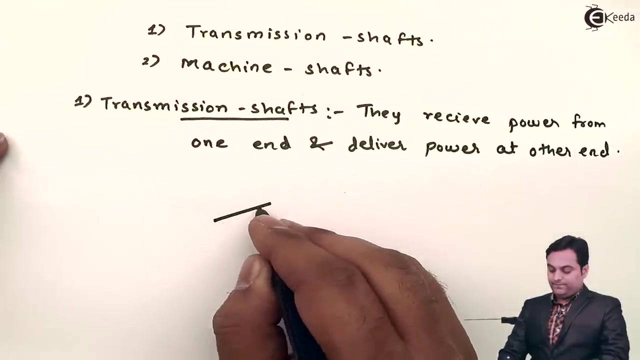 Transmission shafts. they receive power from one end and deliver power at the other end. So, transmission shafts, they receive power and then they even transmit power. if I can explain the transmission shaft with the diagram, then I can show it in this way. here the diagram: 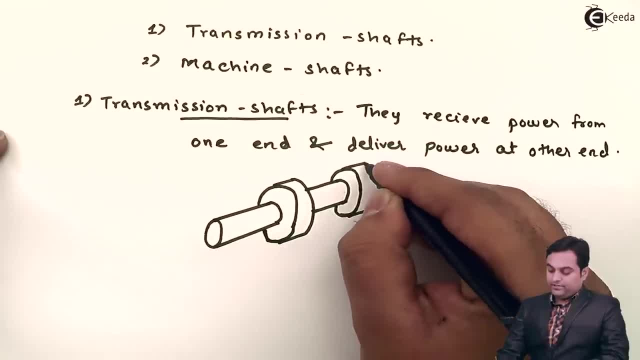 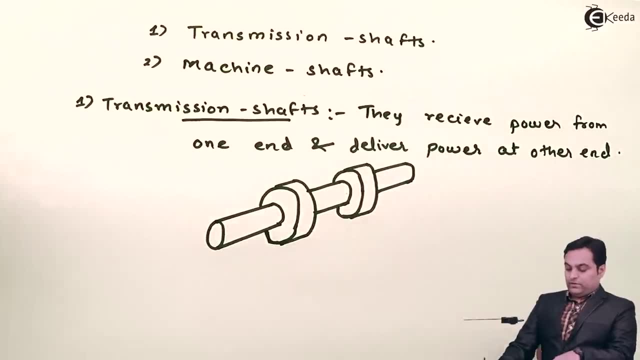 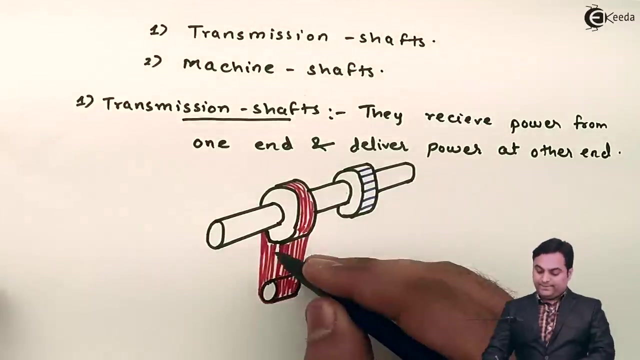 which I am drawing. It means there are some members which are connected. They are kept on this shaft, as we can see in this diagram. Now, in order to rotate this shaft here, suppose we have another pulley which is here Now, here in this diagram, this is the belt which is there on the shaft. 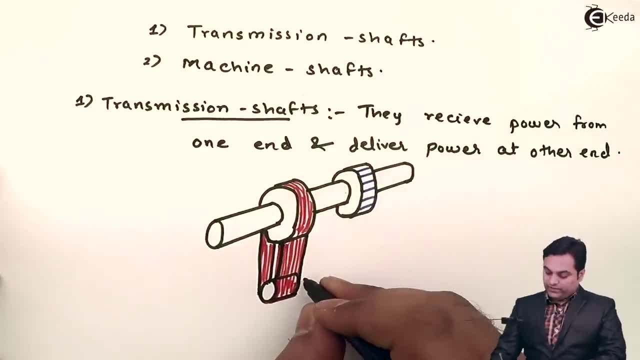 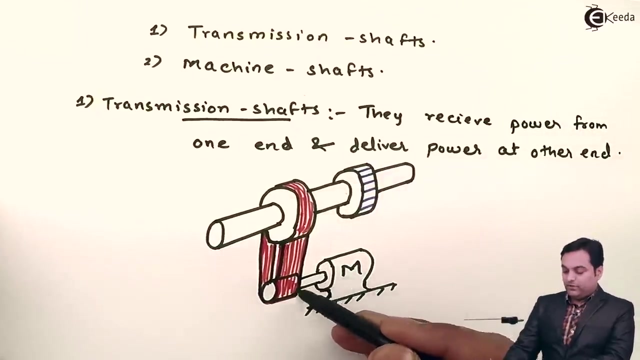 Now how this works, This diagram is. we can understand this in a way that suppose we have some power transmitting device here. this device, I am saying that it is a motor. Now, this motor will transmit power, this shaft will rotate and this smaller pulley would. 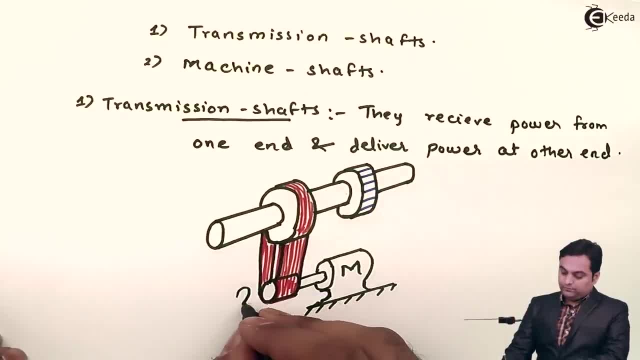 be rotated. This is the help of this motor. now here, as I can see in this red color which I have shown, this is belt and here we have pulley. So when this small pulley, it is rotating, it is receiving power from the motor, which takes 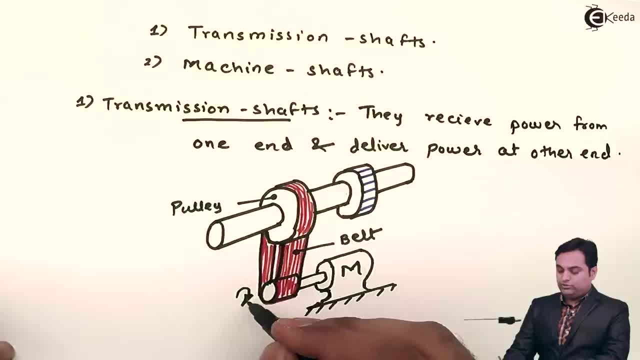 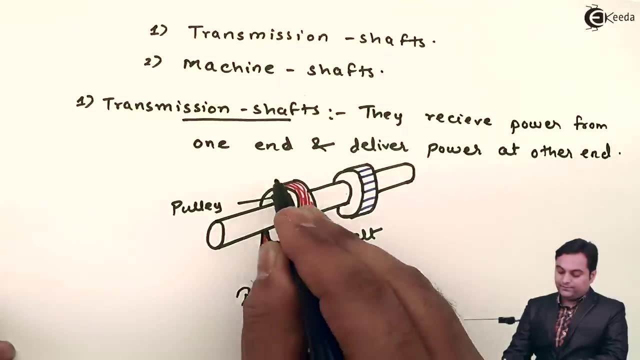 in electrical power and gives mechanical output. So this shaft small pulley is rotating. This small pulley is connected to the bigger pulley with the help of belt, as we can see. So when this rotate, even this bigger pulley rotates with the help of the belt. here in the 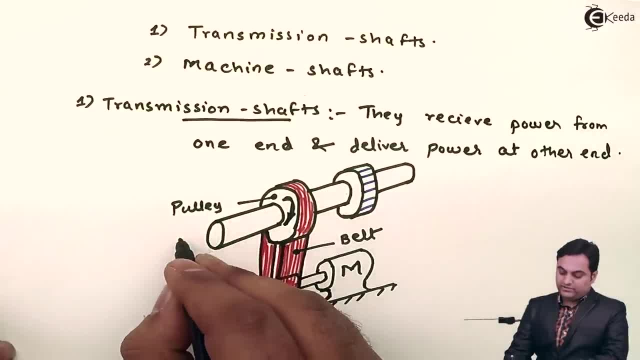 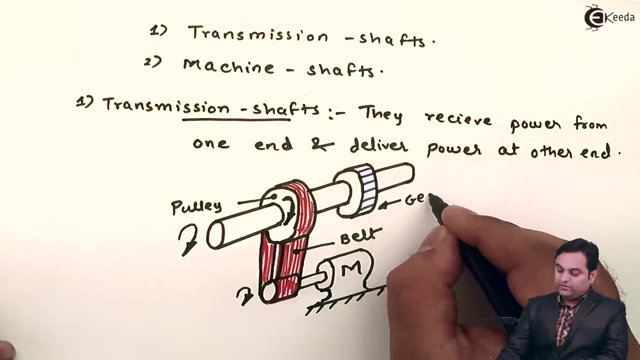 same direction. Now, when this bigger pulley rotates, even this shaft would be rotating in the same direction. So it means we have transferred power from the motor to this shaft. this shaft rotates. Now on this shaft There is another member which is called as the gear like. I am giving you an example of. 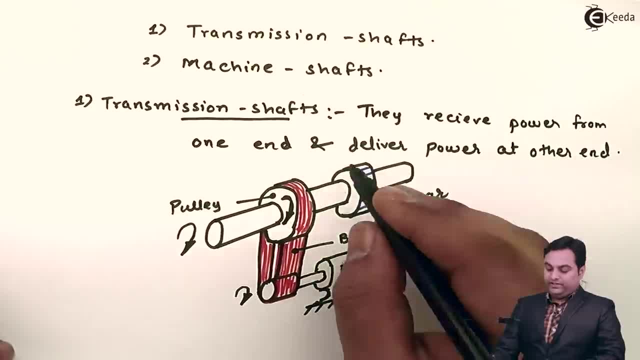 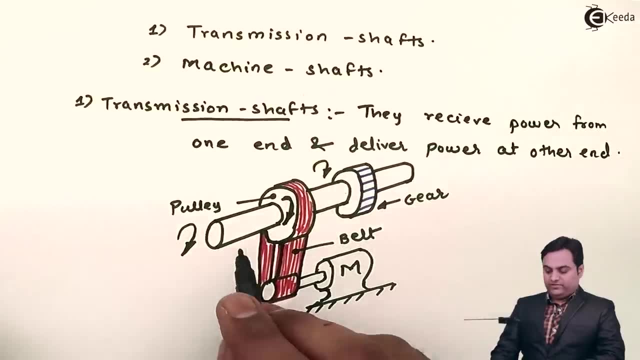 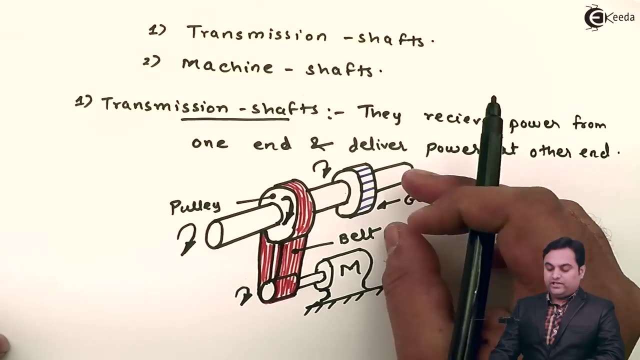 a gear. So this gear also starts rotating into a clockwise direction and, as we can see in this diagram, shaft is receiving power. it is rotating at the same time on this same shaft we are having a gear, and now this gear can be in mesh with another gear, that is, we can make another gear. 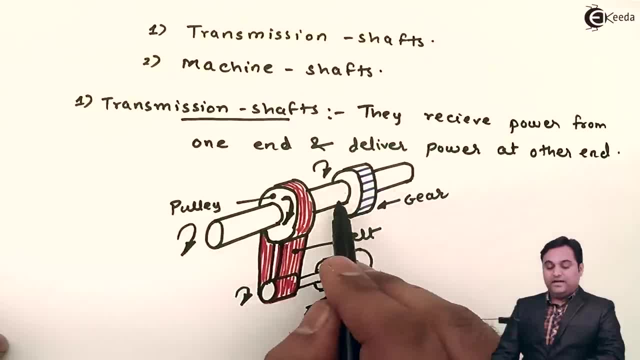 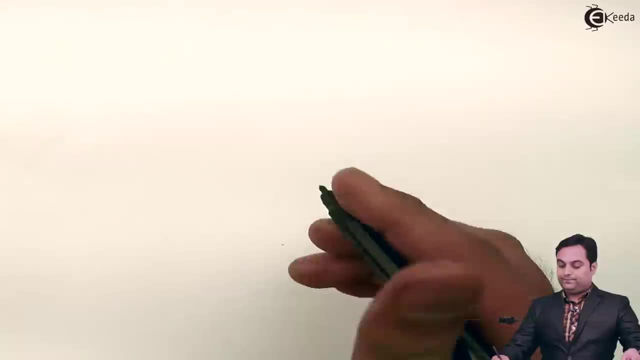 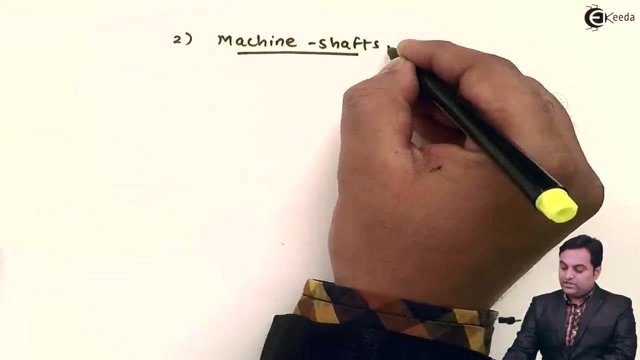 to come in contact with that and that gear would be rotated by this gear. So, as we have seen this shaft, it is receiving power and also it is transmitting power. So there is. this is an explanation of transmission shaft. Now, when we talk about machine shafts- the second type machine shafts- they are an integral 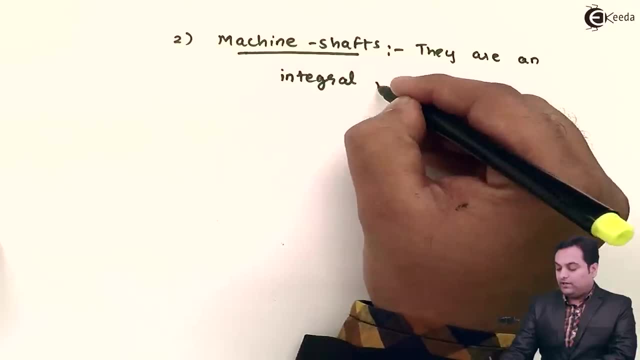 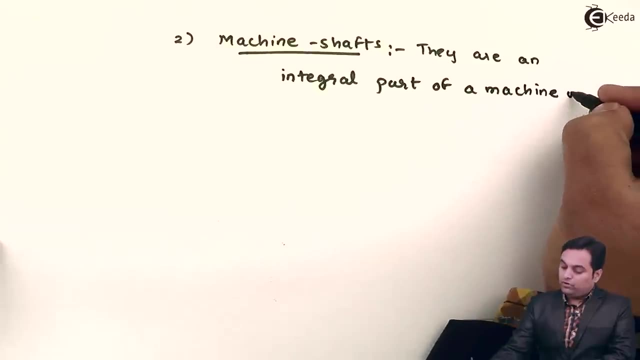 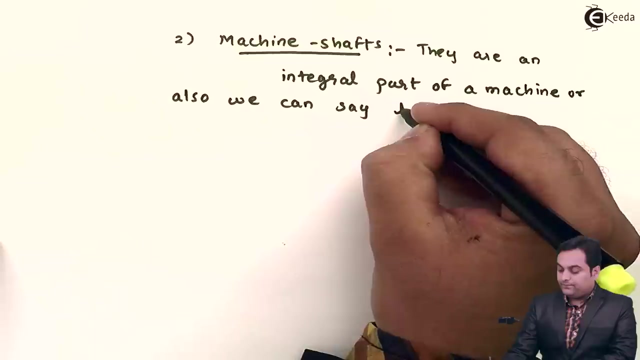 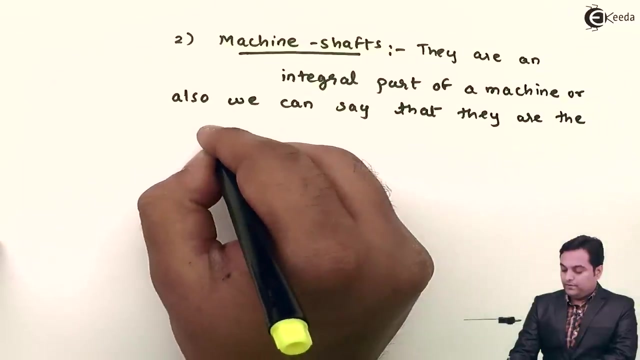 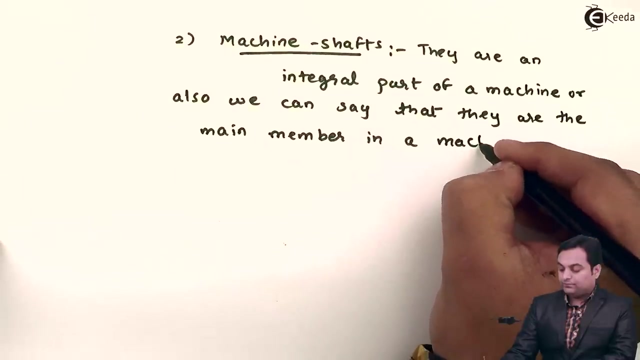 part, So this is an integral part. This is an integral part. This is an integral part, So this is an integral part Of a machine. or also we can say that they are the main member in a machine. I can put the following things above: here we can use a constant, constant, constant. 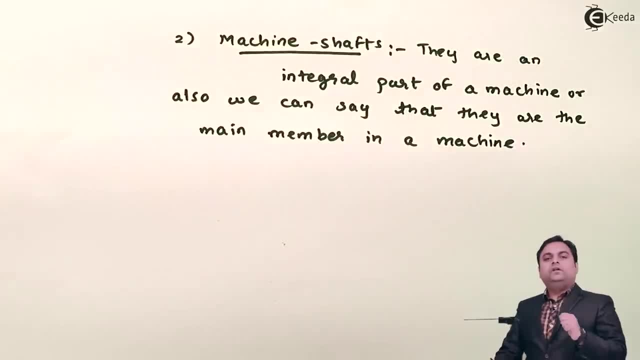 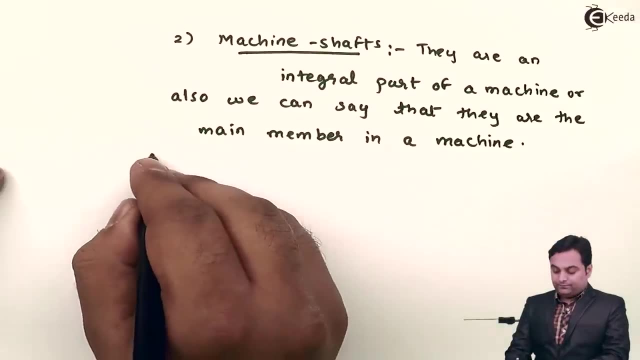 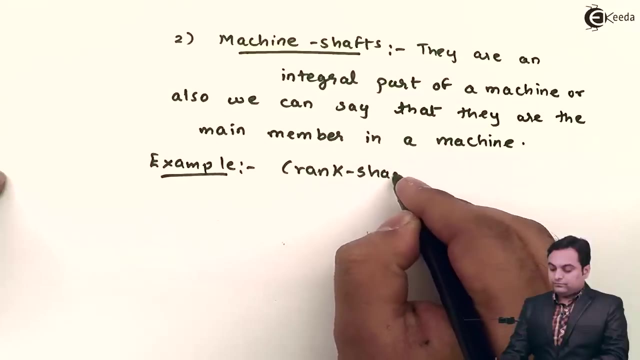 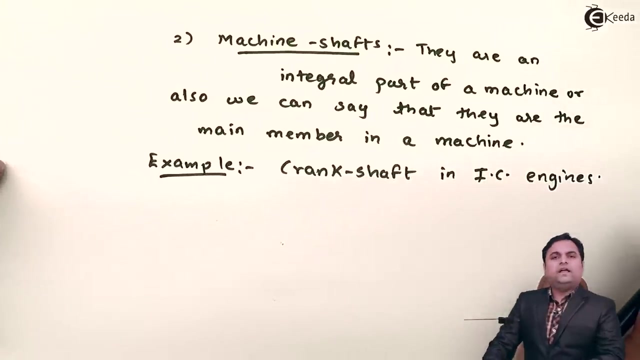 Let us say roommate as well as a machine, as well asك, we can say that they are union members. so here i have written about machine shaft that they are either integral part and also the main part of the machine or main member. example: crankshaft in ic engines, that is, internal combustion engines, so that crankshafts, they are an example of machine. 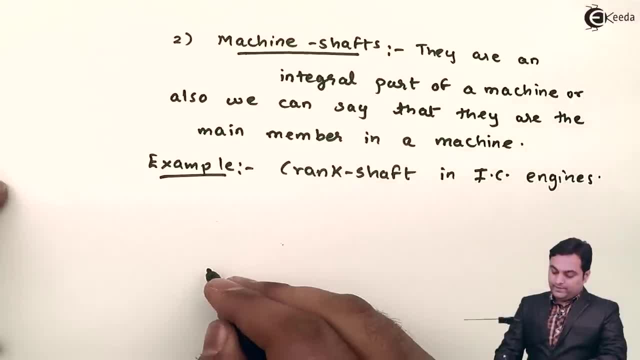 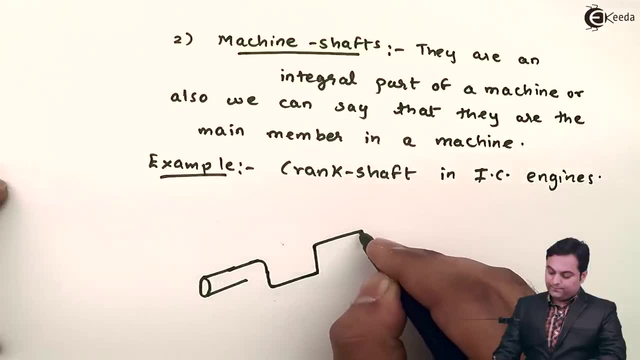 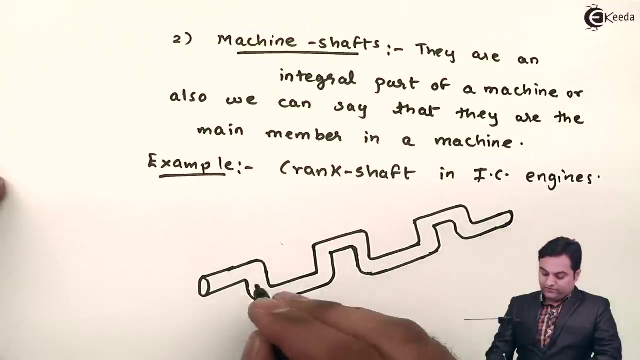 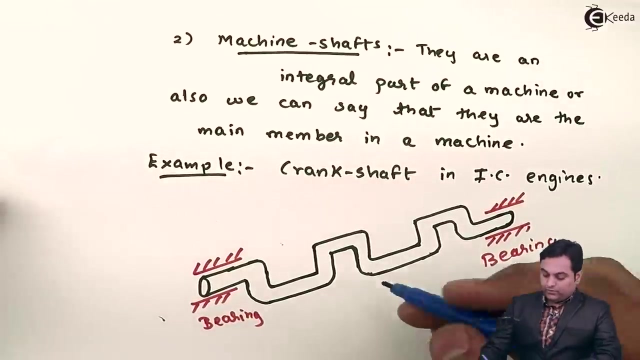 shaft because they are part of the engine and if i can show it with a diagram, crankshaft will look something like this. so here is the diagram of a crankshaft which will be supported in bearings. that is here. if i denote bearing by this symbol, these are the bearing and to this the connecting rod would be joined. 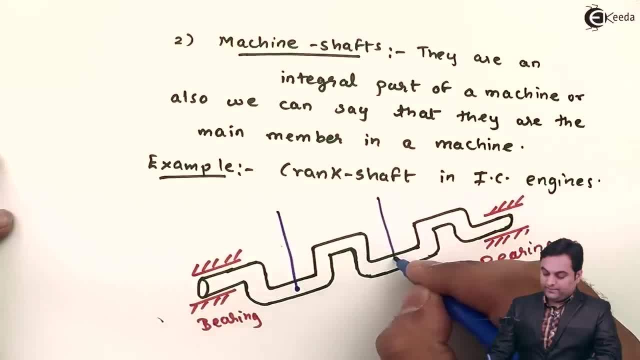 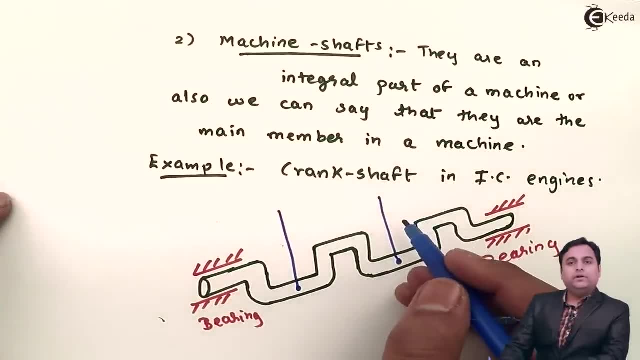 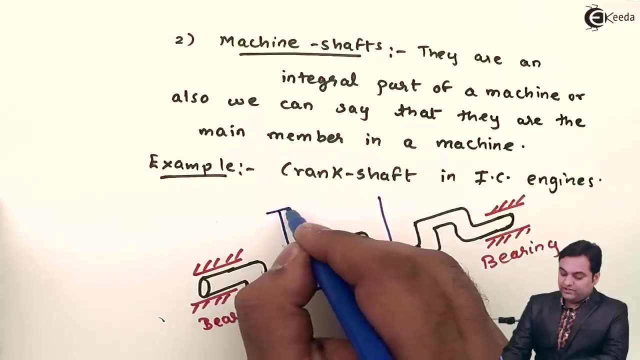 if i am just denoting the connecting rod by a single line. so it means this diagram here. this crankshaft is receiving power. it is receiving power from the connecting rod which is connected to the piston. if i can show them just with the help of a line diagram,